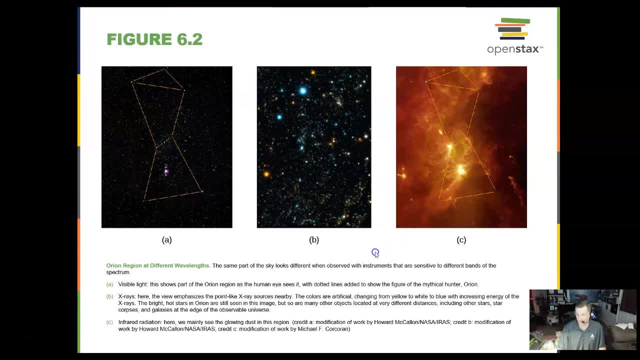 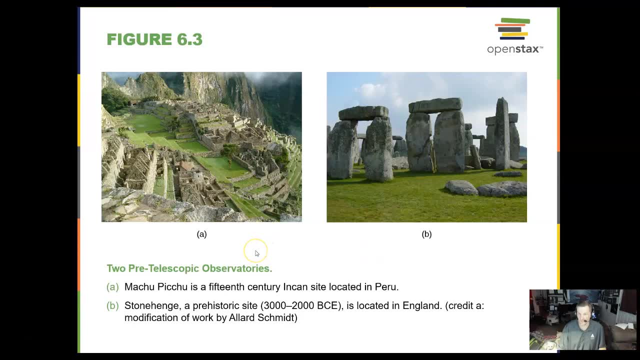 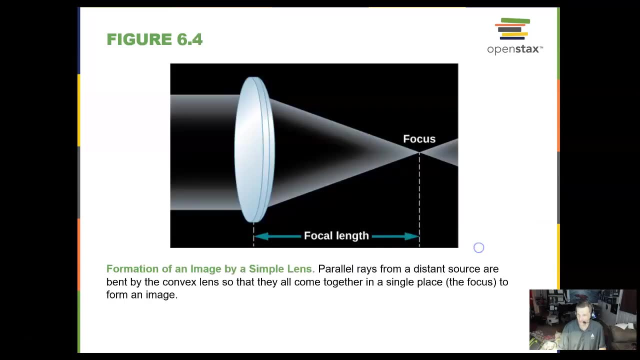 different wavelengths, it looks different ways. Here are two pre-telescopic observatories. One is Machu Picchu in Peru, The other one is Stonehenge in England. The formation of an image by a simple lens has parallel light coming into the lens, being focused, all into a focus point, And that is where you would. 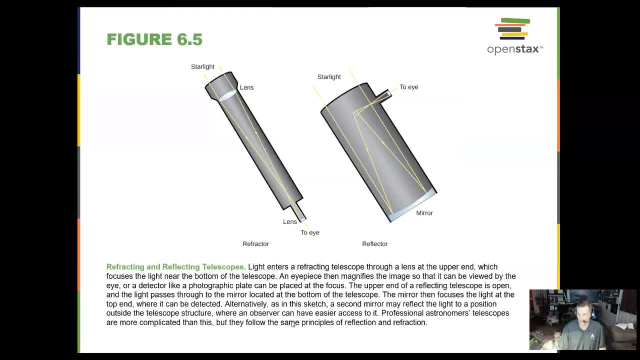 view the image. The difference between refracting telescopes and reflecting telescopes is that, basically, refracting telescopes spin light through a lens, a glass lens, whereas a reflecting telescope reflects light off of a mirror through another mirror that then goes through an eyepiece, which is a lens. 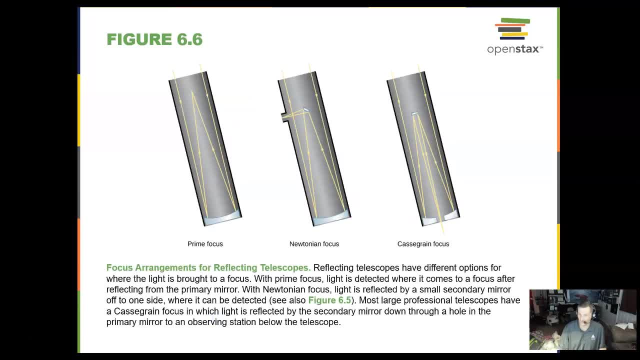 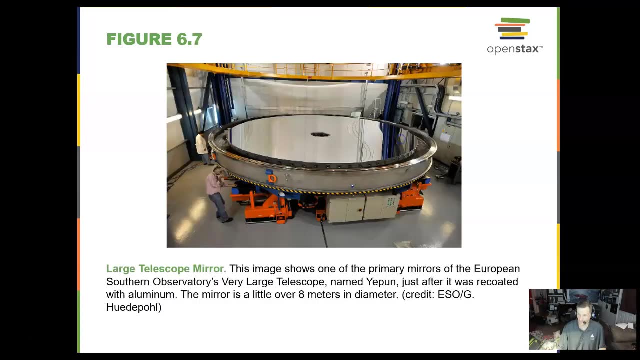 You can have different areas of focus in a reflecting telescope. You can have it coming out of the aperture, the eyepiece or a focus within the mirror itself. Here is a very large telescope mirror. This is going to go on the European Southern Observatory's 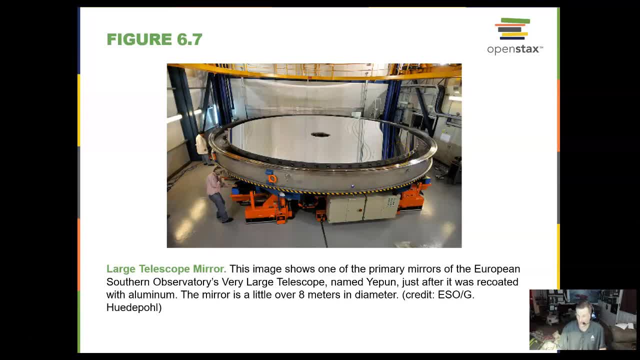 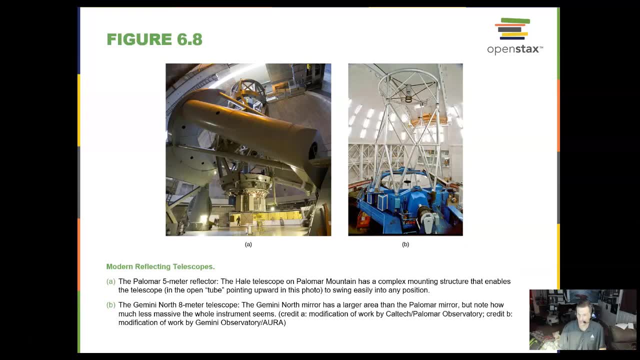 Very Large Telescope. We like to name our instruments and telescopes interesting names. Here are some modern reflecting telescopes: The Palomar 5-meter Reflector which is up here and outside, and the Gemini North 8-meter telescope over here to the right. 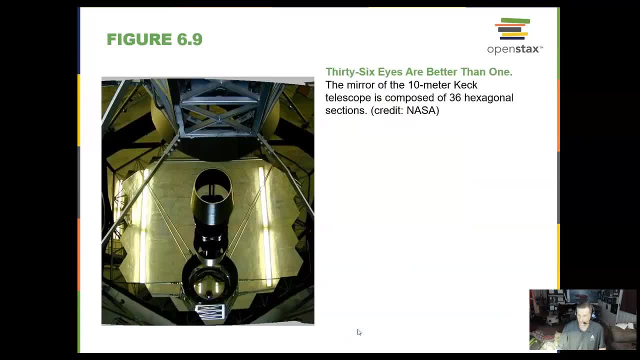 Question: Yes, Yes, Yes, Of course we think that 36 eyes are better than one. In order to build a compact but very large telescope, we can use segmented mirrors. These segments here are all glued together to make one large mirror. This is for Keck Telescope in Hawaii. 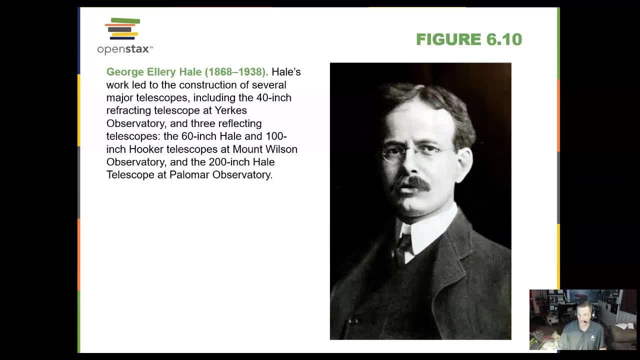 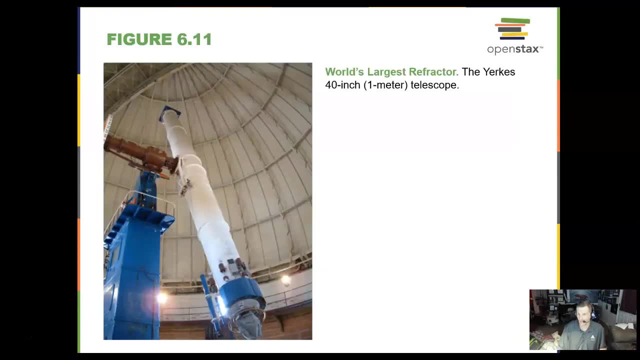 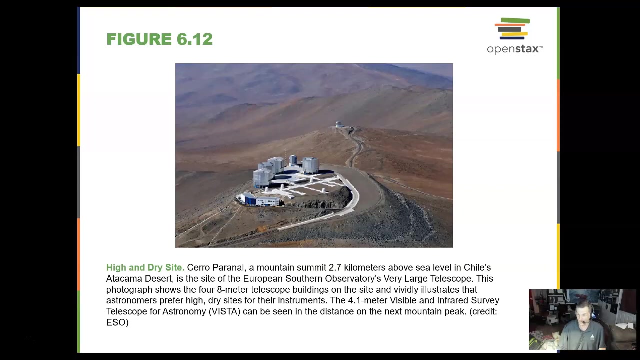 But George Hale led to the work of the construction of several major telescopes. The largest refractor bending telescope in the world is the 40-inch. This is in Chicago. Most observatories are put as far high up on the mountain as they can go. Here we have. 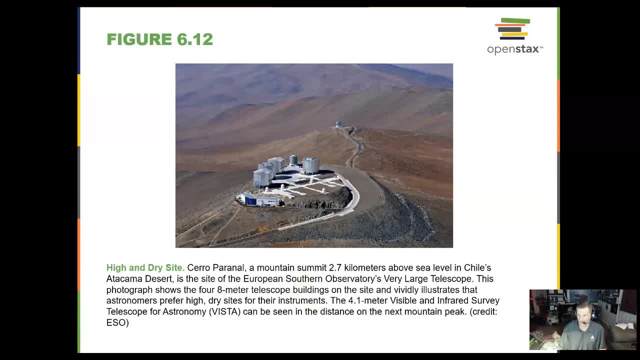 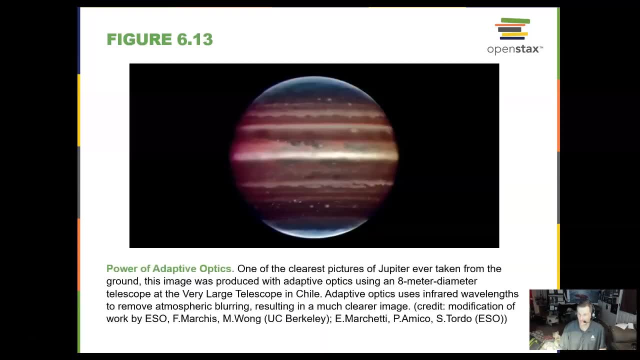 a high and dry site at Chile's Atacama Desert, part of the European Southern Observatory. It's a very large telescope. Here we have a high and dry site at Chile's Atacama Desert, part of the European Southern Observatory. Now we can put pistons on the back of these telescope mirrors and these pistons can move. 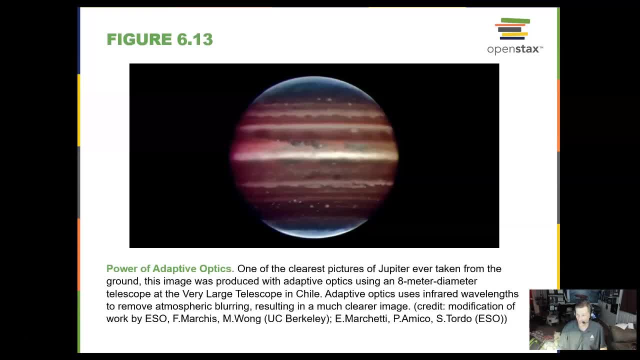 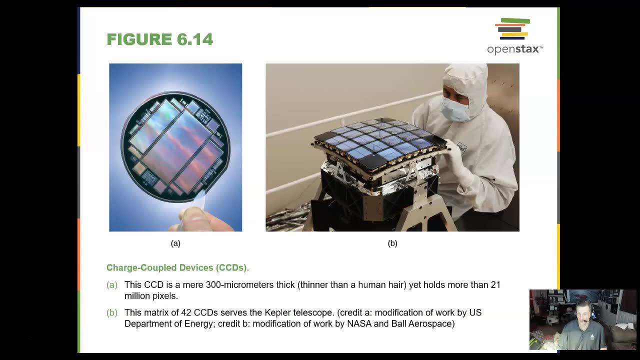 the mirror ever so slightly to correct it for the atmosphere, and that's called adaptive or active optics. So here is a picture of Jupiter with those active optics working and you get a great image. The bed bone of these cameras are these CCDs. they're called charge coupled devices. 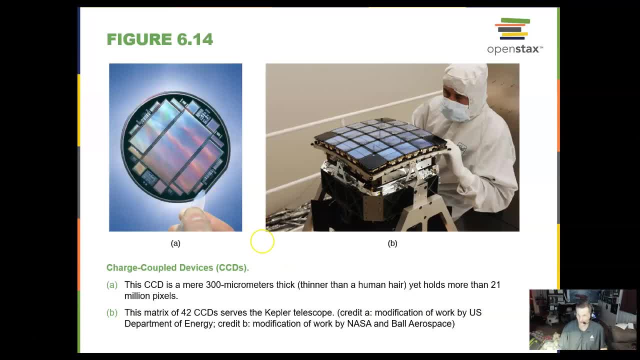 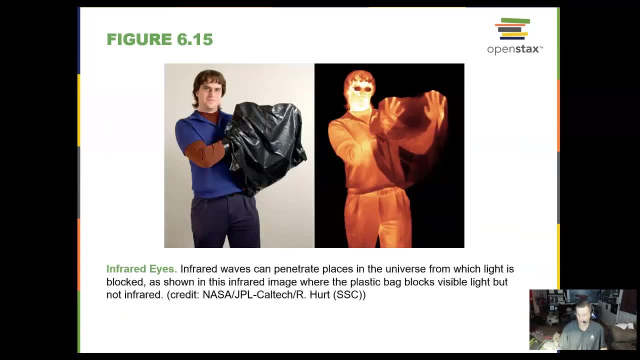 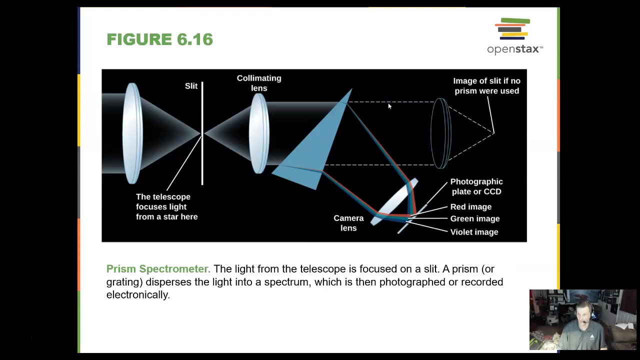 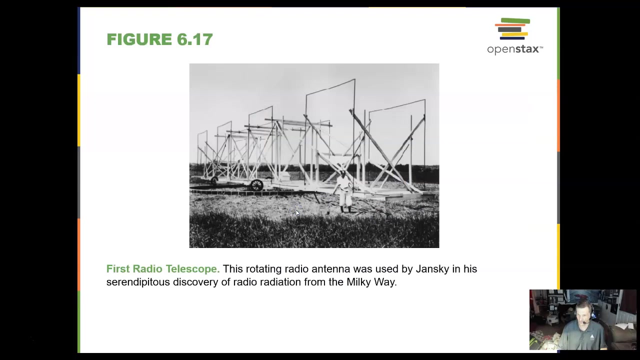 and it's basically a silicon wafer that is sensitive to light. In the infrared we can see these hands in the bag very clearly in the infrared. Infrared gives off heat radiation. In a prism spectrometer, this is an instrument that will split up the light from white light into its colorful rainbow pattern. Here's the first radio telescope. 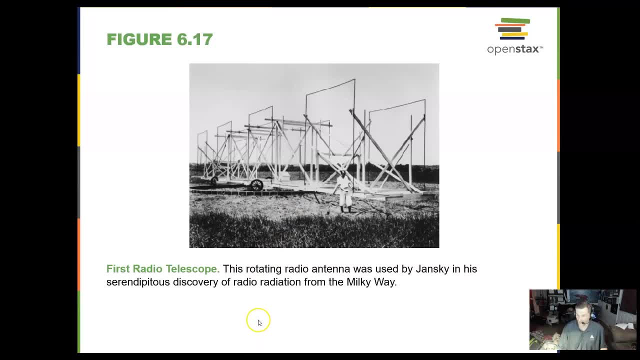 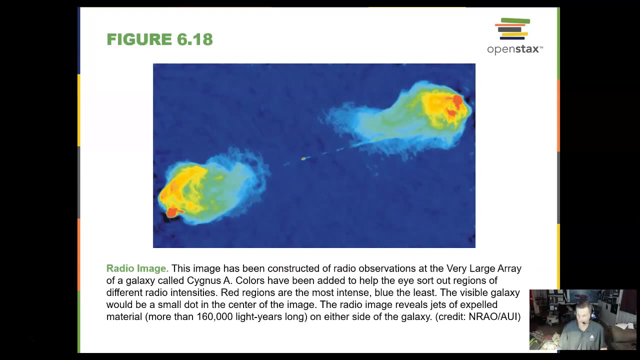 very basic. This telescope was used by Jansky in his discovery of radio radiation from the Milky Way. This is what a radio image looks like. There is a galaxy right here in the middle that doesn't give off very much radio information, but coming off two lobes out far out in space. we see jets coming from this image. 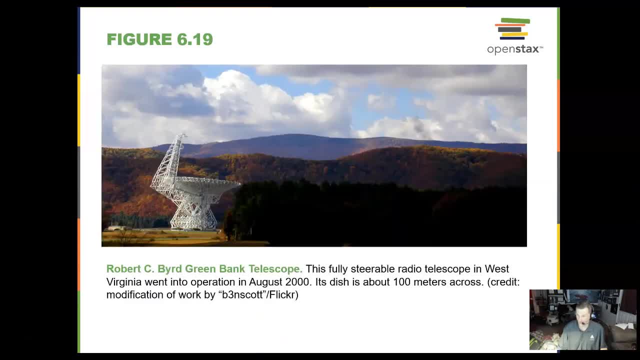 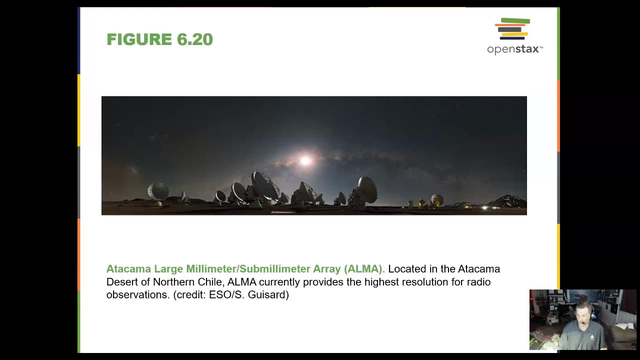 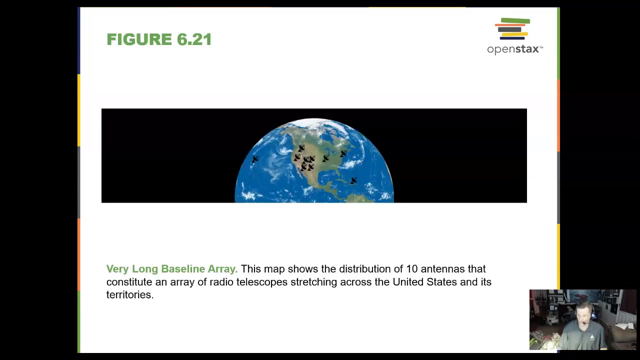 The Green Bank Telescope in West Virginia is pretty large, 100 meters across The Large Millimeter Array in Chile, the Atacama Desert again in northern Chile. Or you can put radio telescopes throughout the earth and link them all together so that the earth is. 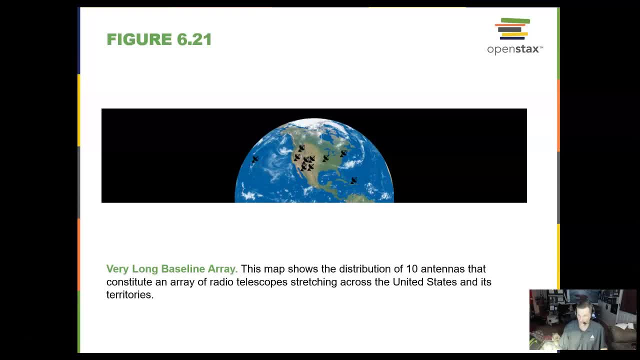 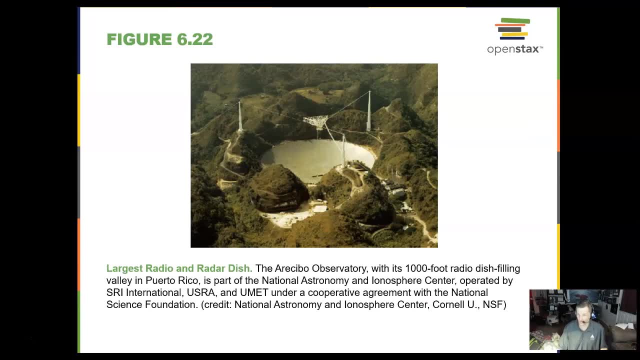 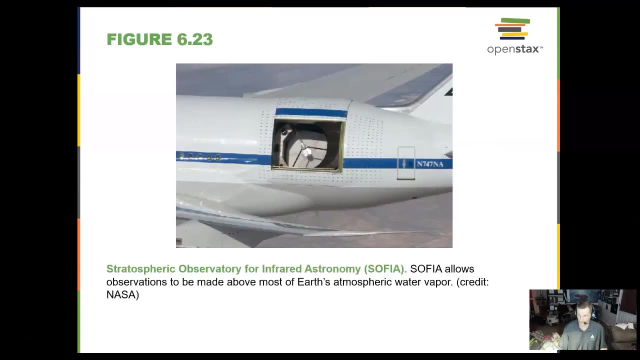 acting like a radio dish, the entire earth. The largest radio and radar dish in the world is the Arecibo Observatory in Puerto Rico. We can put observatories into the upper atmosphere- SOFIA allows us to do that- and get above most of the earth's water vapor, which 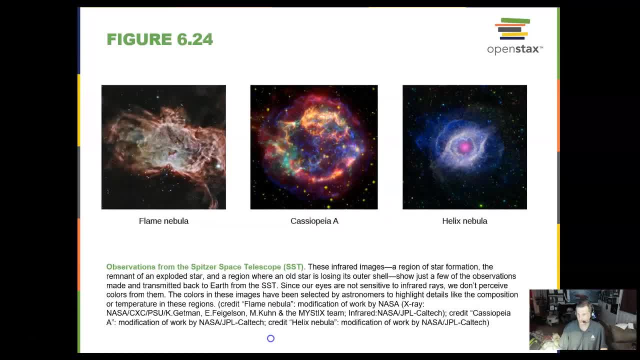 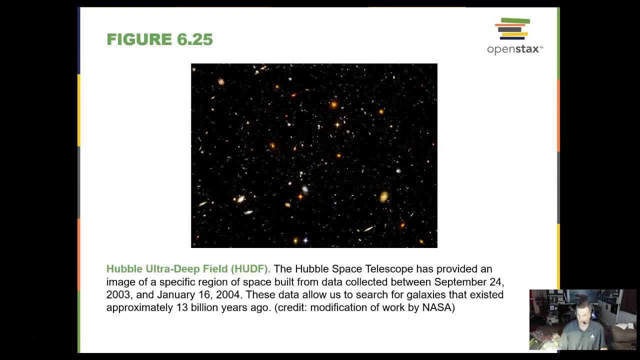 is blinding to infrared light. The Spitzer Space Telescope does infrared images like these, And then we have images like this. This is the Hubble Ultra Deep Field, And this is an area of space that we can go back into 13 billion years ago, when 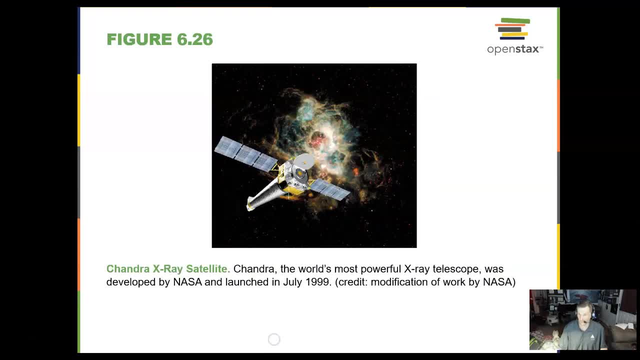 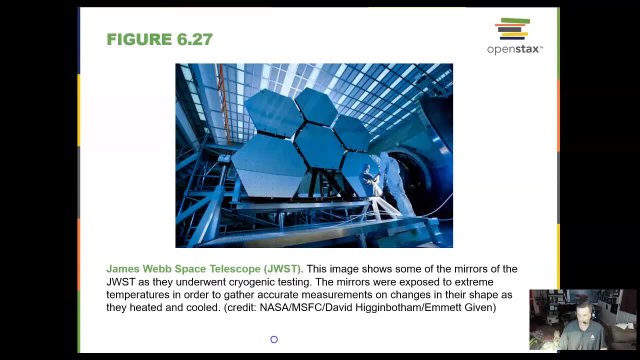 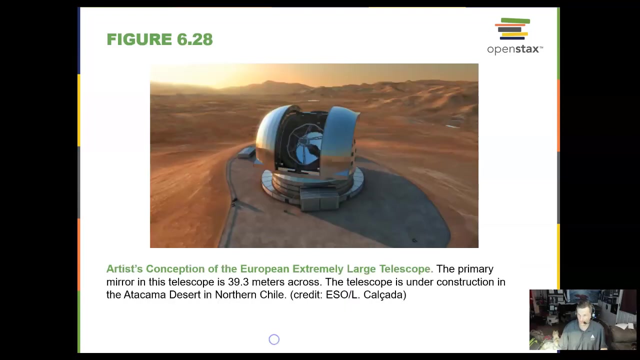 it was formed by looking back into time. The Tandra X-ray Satellite does the same thing, but for X-rays, And then, coming up in 2021, is the James Webb Space Telescope to be launched, And it's going through some very rigorous testing right now. 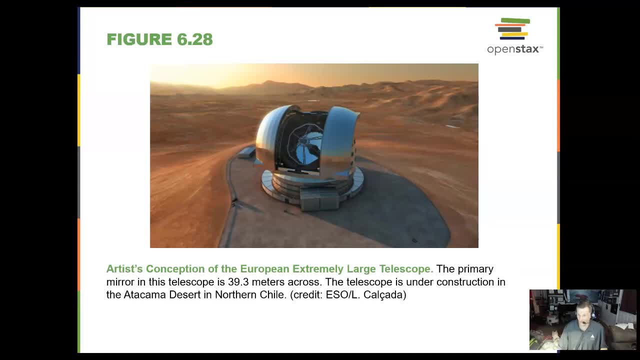 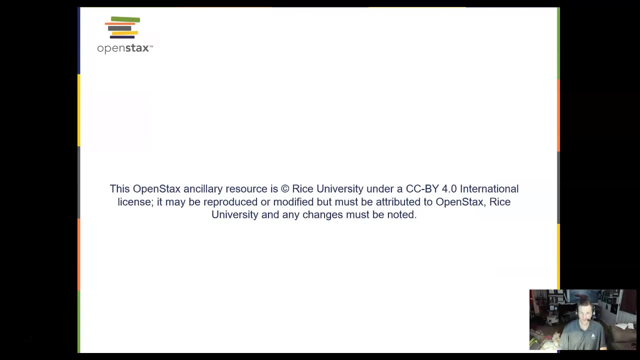 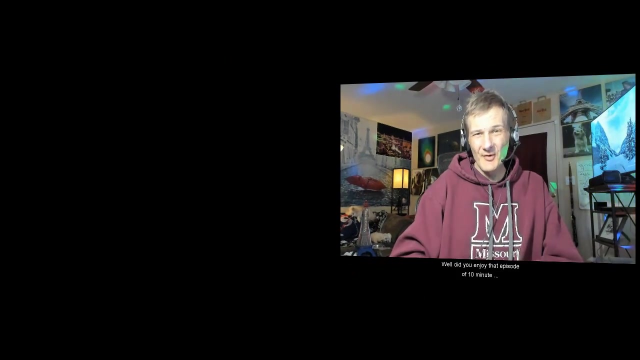 And then the European Extremely Large Telescope. It will be almost 40 meters across, And this is currently under construction in Chile. Thank you for joining us for Chapter 6.. Well, did you enjoy that episode of 10-Minute Astronomy? 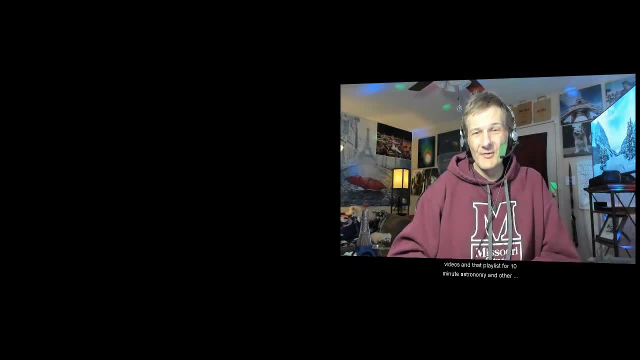 If so, check out all the other videos in that playlist for 10-Minute Astronomy and other videos on my channel, and then hit the subscribe button right there. Thanks,